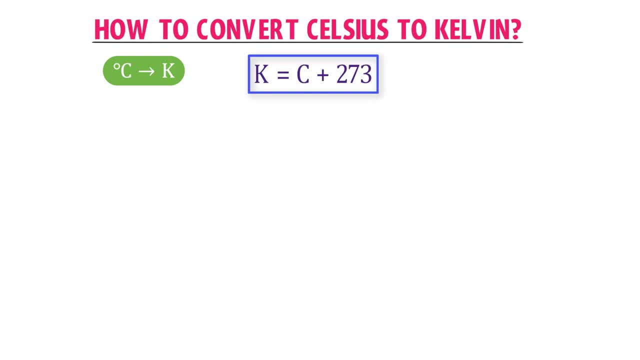 is K is equal to C plus 273.. Here K is the Kelvin temperature and C is the Celsius temperature. Now, for example, convert 40 degree centigrade to Kelvin temperature. I will just plug in this 40 degree centigrade. in this formula K is equal to 40 plus 273.. Now 40 plus 273 is equal to 313. 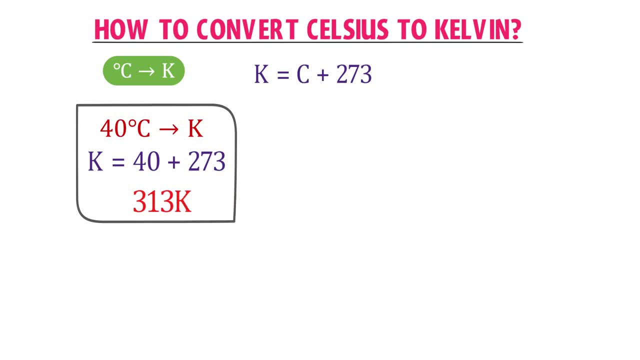 Thus I get 313 Kelvin Here. the easiest trick of converting any Celsius temperature to Kelvin temperature is by adding 273 to the Celsius temperature. I mean always: add 273 to Celsius temperature and you will get Kelvin temperature. Now how to convert Kelvin temperature to Celsius temperature or degree centigrade. 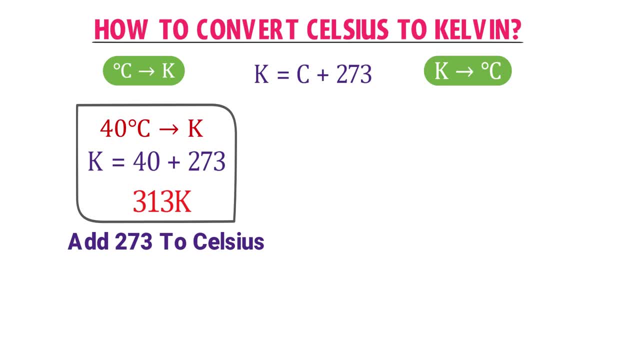 We know that the formula of this conversion is: K is equal to C plus 273.. Let's consider that. convert 313 to Kelvin temperature. Now, how to convert Kelvin temperature to Celsius temperature? We know that the formula of this conversion is: K is equal to C plus 273.. Let's consider that. 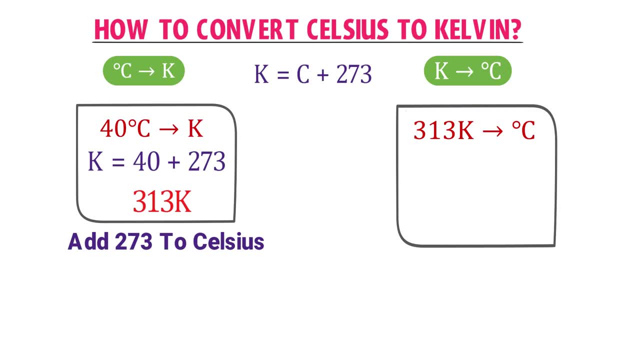 convert 313 to Delta degrees, equal to 313 Kelvin to degree centigrade or Celsius. Now, Instead of this K, I will put this 313 Kelvin temperature. I get 313 is equal to C plus 273.. Shift this 273 from the right hand side to the left hand side. 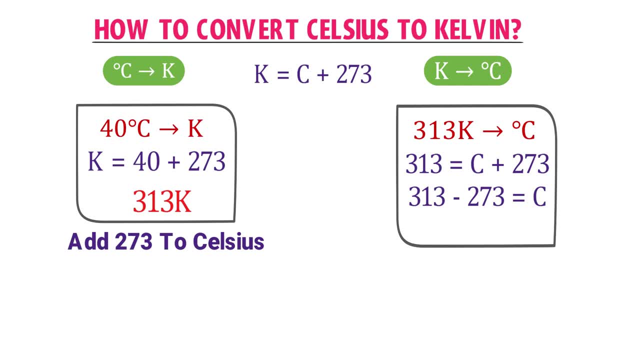 I get. 313 minus 273 is equal to 310 Kelvin максимum temperature. Now I will use this Canvas classroom Kelsey, which is equal to 40 degree centigrade. Here we also learn the trick: always subtract 273 from the Kelvin temperature and you will get. 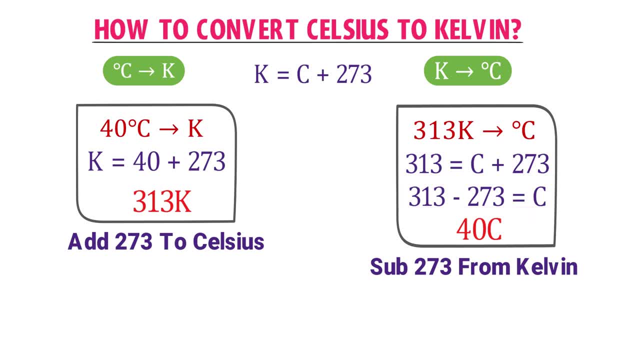 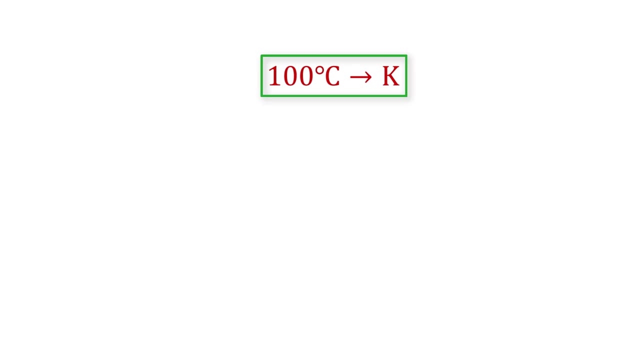 the Celsius temperature. Thus we learn two easiest tricks for this conversion. Let me teach you that, how quickly you can use these two tricks. For example, convert 100 degree centigrade temperature to Kelvin temperature. Here let me also teach you my personal mnemonic which. 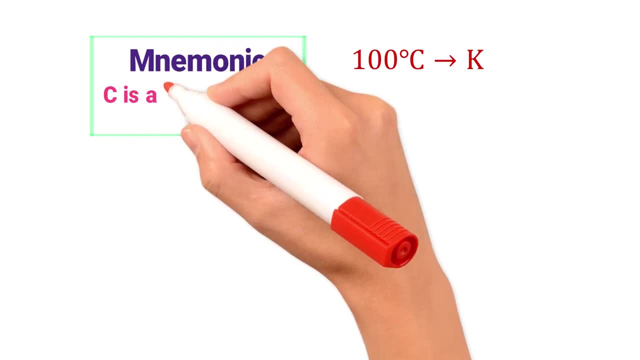 I always teach to my students Here: C is a small cat, while K is a big kangaroo. Small cat C needs our support, while big kangaroo doesn't need any support. C needs our support. hence add 273 to C. I get 373 Kelvin. Thus, 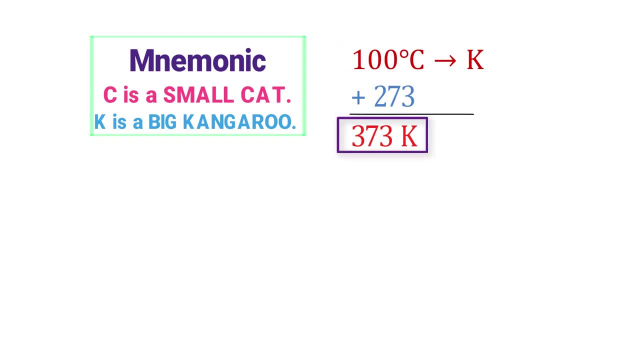 100 degree centigrade is equal to 373 Kelvin. Therefore, always add 273 to degree centigrade or degree Celsius when you convert it to Kelvin temperature. The another example is convert 150 degree centigrade to Kelvin. Here C is small cat It. 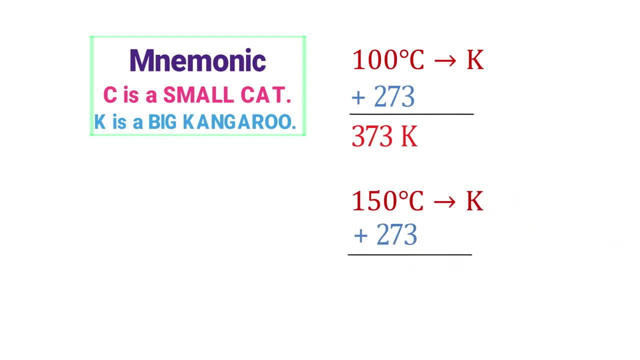 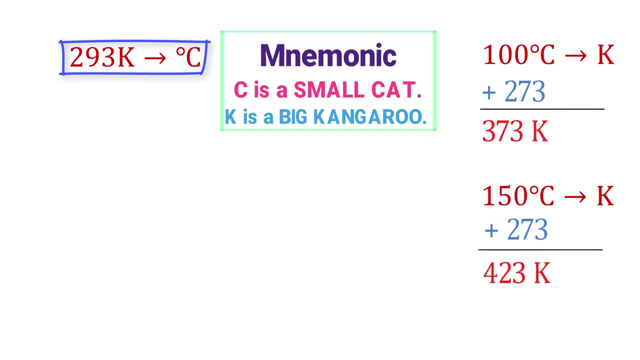 needs our support. Add 273 to this small cat C, we get 423 Kelvin. Thus 150 degree centigrade is equal to 423 Kelvin. Now how can you convert Kelvin to Celsius temperature? For example, convert 293 Kelvin to degree Celsius. This K is big. 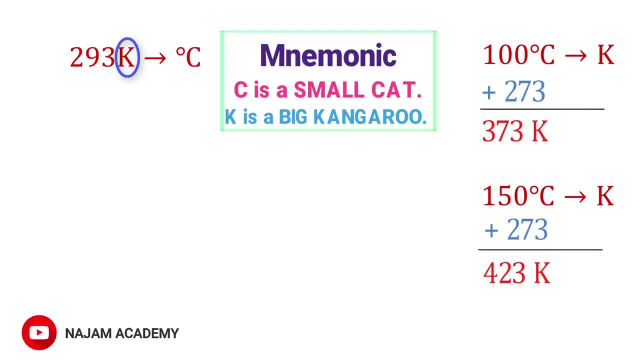 kangaroo, it doesn't need any help or support. Subtract 273 from it, We get 20 degree centigrade. Thus 293 Kelvin is equal to 20 degree centigrade. One another example is convert 388 Kelvin to degree Celsius temperature. 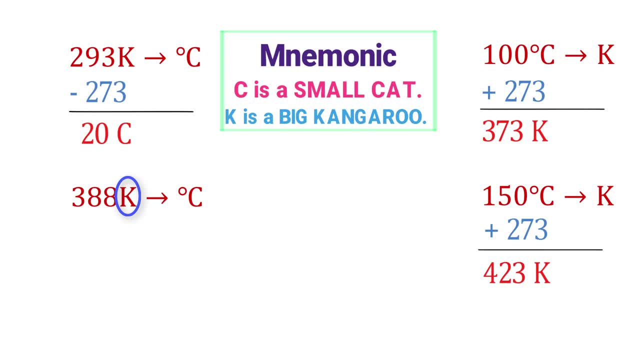 Here. this K is again a big kangaroo. It doesn't need our help or any support. Subtract 273 from it And we get 115 degree centigrade. Thus 388 Kelvin is equal to 115 degree centigrade, Hence. 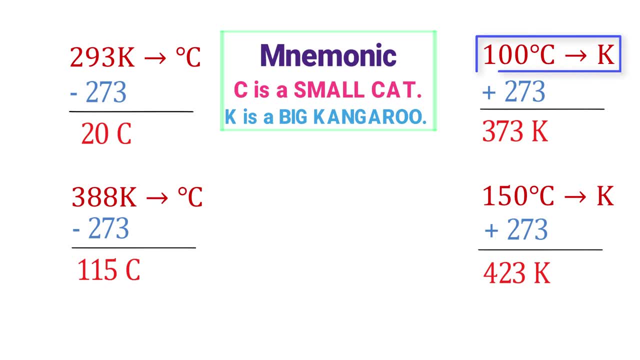 remember that when you convert Celsius temperature to Kelvin temperature, always add 273 to it, While if you convert Kelvin temperature to Celsius temperature, always subtract 273 from it. I hope that you have learnt these tricks of temperature conversion. Now let me teach you that. how do you calculate? 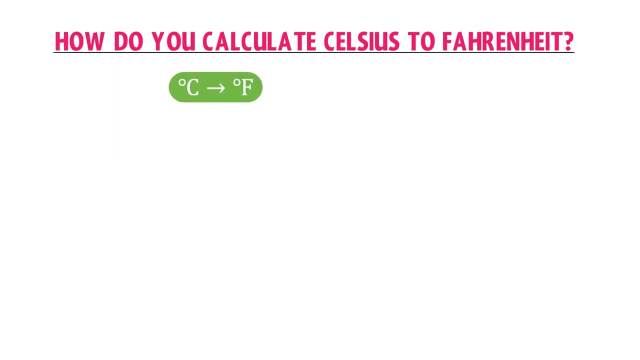 Celsius to Fahrenheit or degree centigrade to Fahrenheit. The formula of this conversion is: F is equal to 1.8 C plus 32, where F is Fahrenheit temperature and C is Celsius or centigrade temperature. For example, convert 12 degree centigrade. 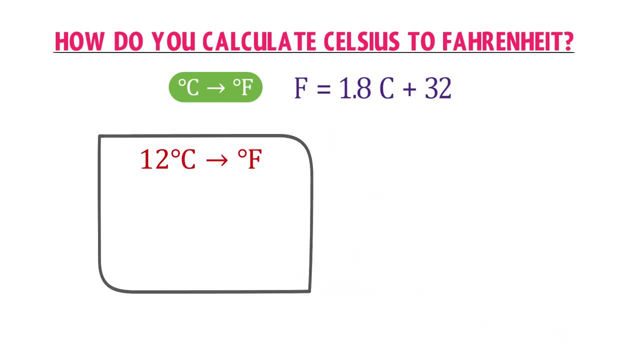 to degree Fahrenheit. Well, I am given temperature in Celsius or in degree centigrade. Thus I will put or plug in this 12 degree centigrade. in this formula, instead of this C, I get F is equal to 1.8 into. 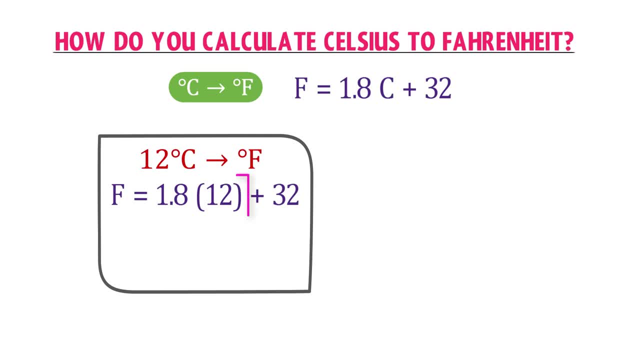 12 plus 32.. 1.8 into 12 is equal to 21.6.. Thus I write, F is equal to 21.6 plus 32.. As a result, I get 53.6 degree Fahrenheit, Therefore 12 degree centigrade. 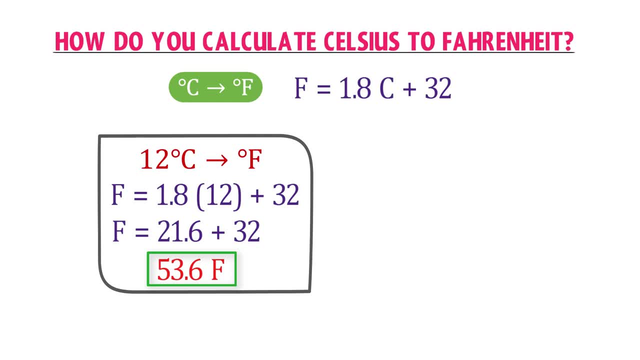 is equal to 53.6 degree Fahrenheit. Let me give you one another example of conversion. Convert 50 degree centigrade to degree Fahrenheit. We know that the formula of this conversion is: F is equal to 1.8 C plus 32.. 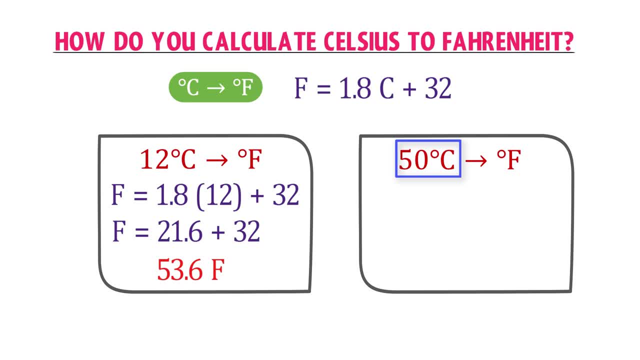 Put the 50 degree centigrade temperature instead of this C in this equation Here. F is equal to 1.8 into 50 plus 32.. 1.8 into 50 is equal to 90.. I write: F is equal to 90 plus 32.. 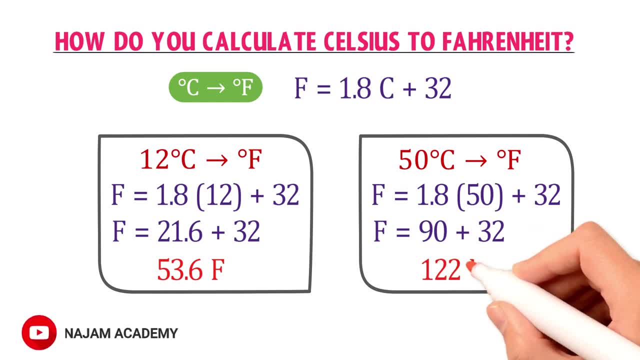 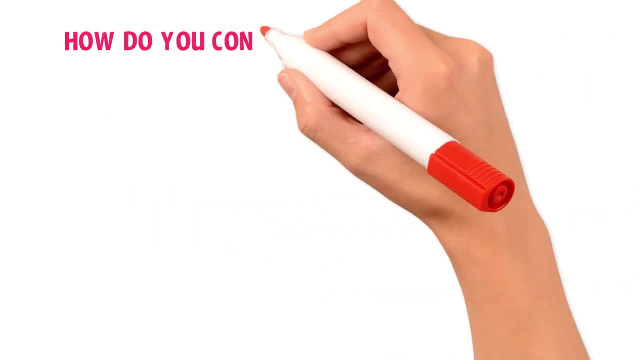 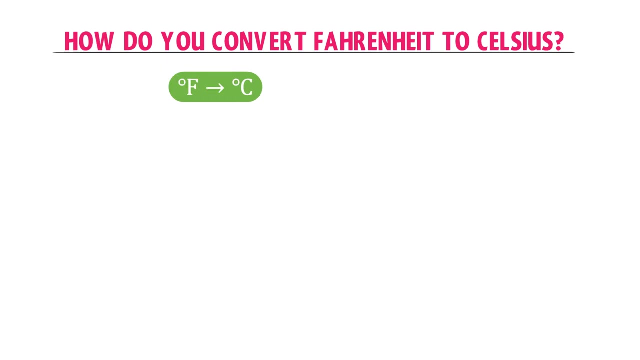 As a result, I get 122 degree Fahrenheit temperature. Thus, 50 degree centigrade temperature is equal to 122 degree Fahrenheit temperature. Now let me teach you that. how do you convert Fahrenheit to Celsius or degree Fahrenheit to degree centigrade? We already know that the formula of 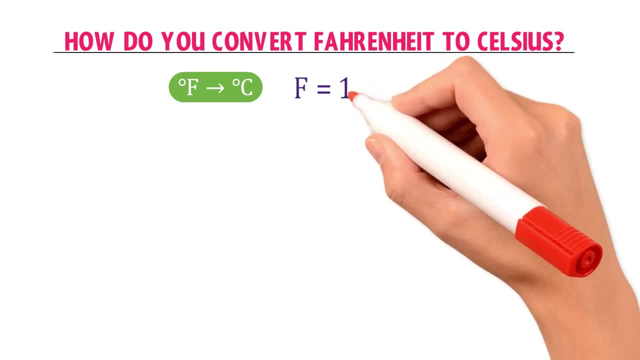 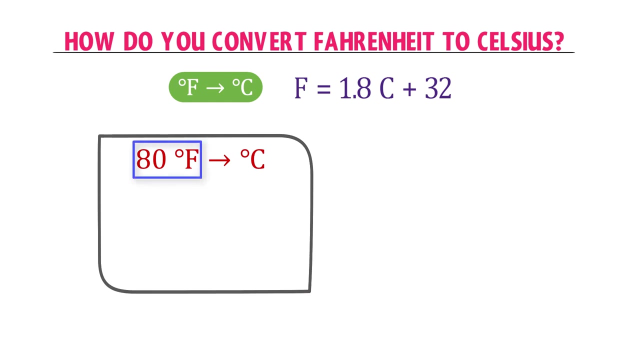 this type of conversion is: F is equal to 1.8 into C plus 32.. Now consider that. convert 80 degree Fahrenheit to degree centigrade. I will put this 80 degree Fahrenheit in this formula I get 80 is equal to. 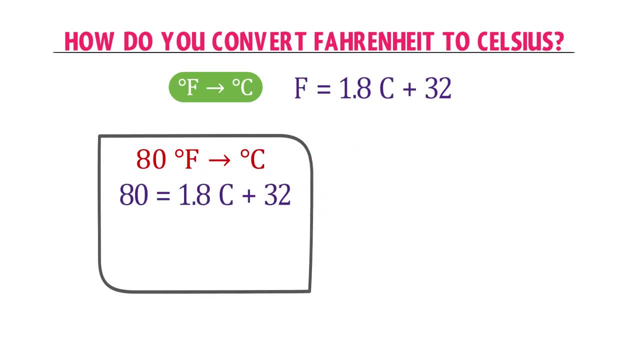 1.8 into C plus 32.. Shift this 32 from the left hand side. 80 minus 32 is equal to 1.8 into C. 80 minus 32 is equal to 48.. Now, dividing both sides by: 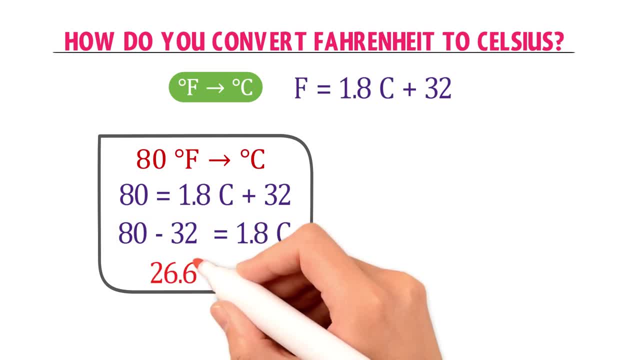 1.8.. I get 26.67 degree centigrade. Thus 80 degree Fahrenheit is equal to 26.67 degree centigrade. Now the another example of such type of conversion is convert 120 degree Fahrenheit to degree centigrade, or. 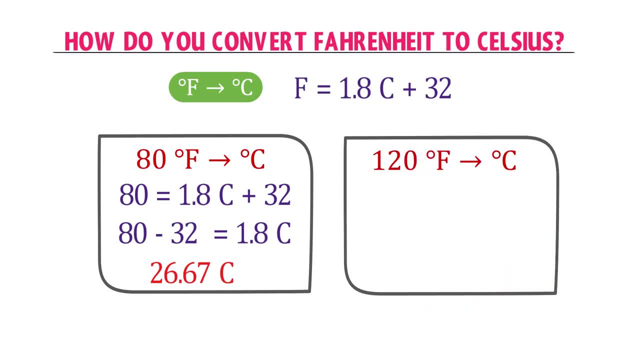 degree Celsius. We know that the formula is: F is equal to 1.8 into C plus 32.. Thus plug in this value and this equation: 122 is equal to 1.8 into C plus 32.. Shift this 32 from the left hand side. 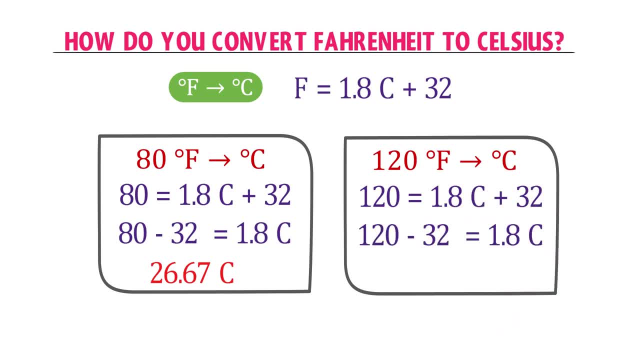 122 minus 32 is equal to 1.8. into C: 122 minus 32 is equal to 88.. Now dividing both sides by 1.8. I get 48.8 degree centigrade. Thus, 122 degree Fahrenheit is equal to. 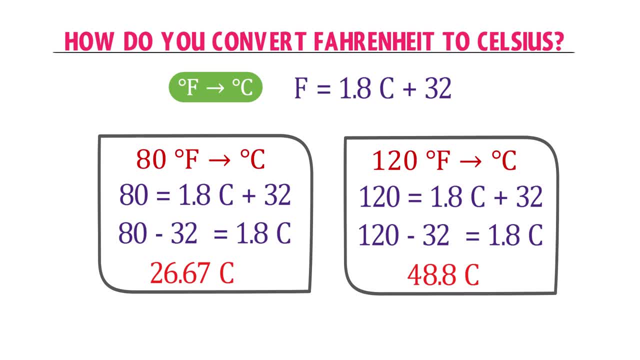 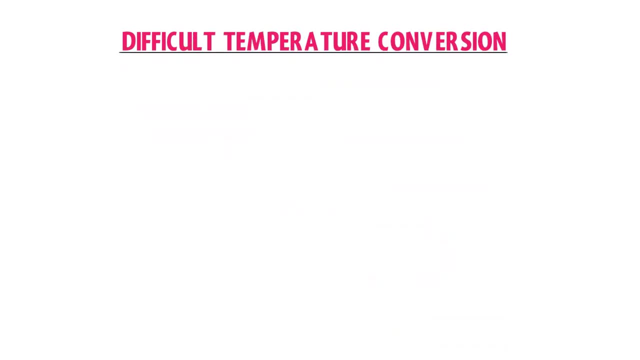 48.8 degree centigrade. I hope that you have learned the Celsius, or centigrade, and Fahrenheit temperature conversion At last. let me teach you a difficult conversion of temperature. Consider 300 Kelvin temperature. Now, if I ask you convert this 300 Kelvin temperature, 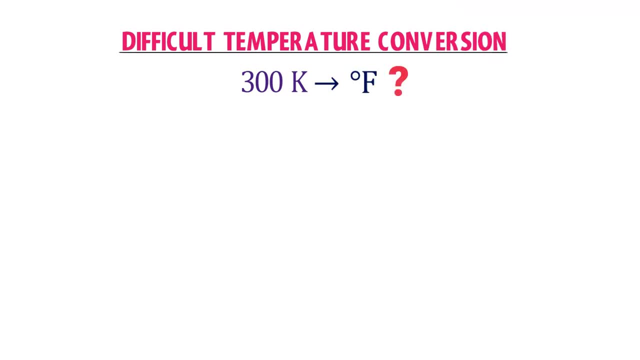 to degree Fahrenheit. Will you convert it? I hope you can. Let me calculate it for you. Firstly, I will convert this 300 Kelvin temperature to degree centigrade and then I will convert degree Celsius to degree Fahrenheit. By this way I will convert. 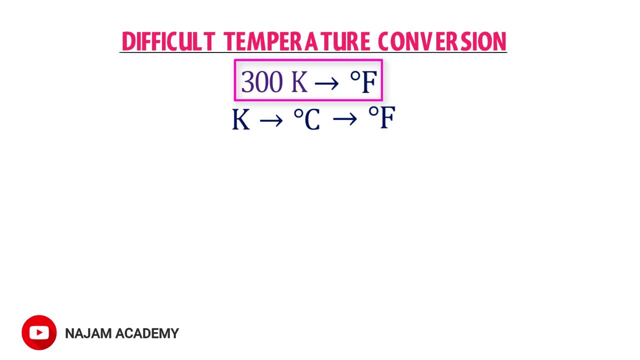 this Kelvin temperature to degree Fahrenheit temperature, Thus first convert 300 Kelvin to degree Celsius. Again, we use the mnemonic we learnt previously. Here K is a big kangaroo, It doesn't need our support. Thus subtract 273 from this K, our kangaroo. 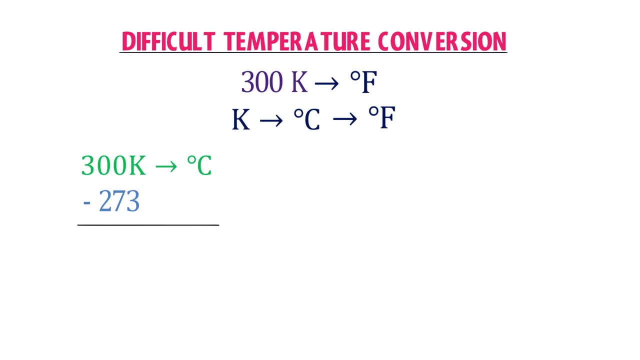 300 Kelvin minus 273, I get 27 degree centigrade. Now I will convert this 27 degree Celsius to degree Fahrenheit. We know that the formula of Celsius and Fahrenheit conversion is: F is equal to 1.8 into C plus 32.. 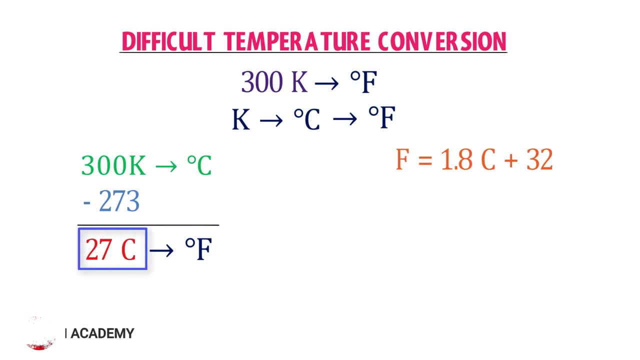 We will plug in this 27 degree centigrade. in this equation, F is equal to 1.8 into 27 plus 32.. 1.8 into 27 is equal to 48.6.. I write: F is equal to. 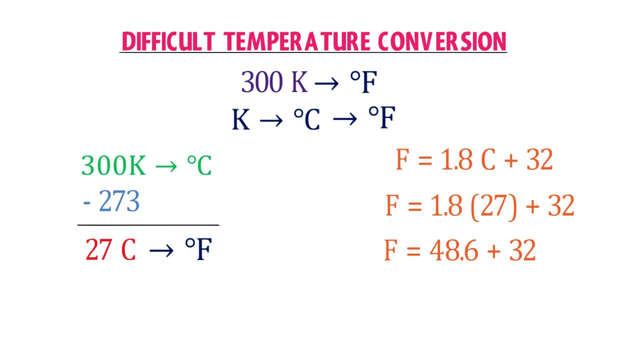 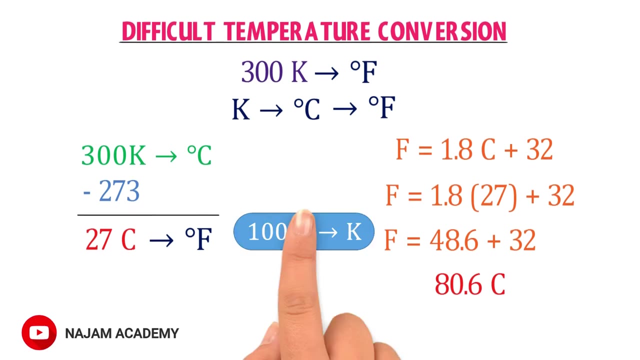 48.6 plus 32.. As a result, I get 80.6 degree Fahrenheit. Thus 300 Kelvin is equal to 80.6 degree Fahrenheit. Finally, convert 100 degree Fahrenheit to Kelvin and drop your answer in the comment box. 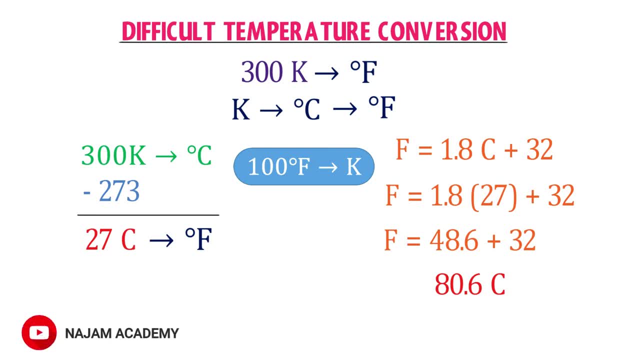 This was all about temperature conversion. If you have learned something new in this video, then like this video and subscribe our channel for more conceptual lectures. Thank you very much for watching this video.